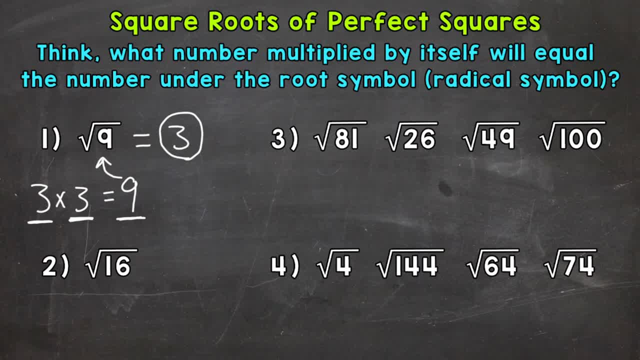 So we need to think again what number multiplied by itself equals 16.. We know 4 times 4 equals 16.. 4 times 4 equals 16.. So a number multiplied by itself gives us the number under the square root symbol. 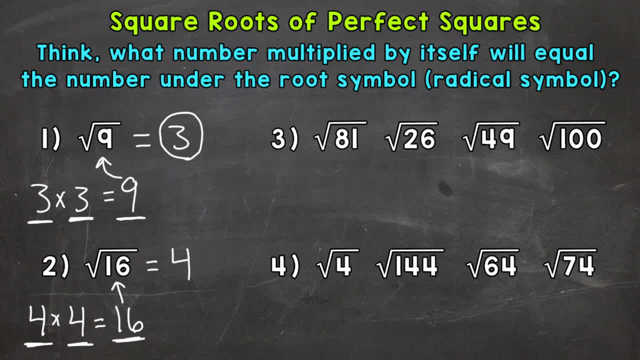 So the square root of 16 equals 4.. And that's our final answer. Let's move on to numbers 3 and 4, where we have 4 square roots for each. 3 of the 4 will have square roots of perfect squares. 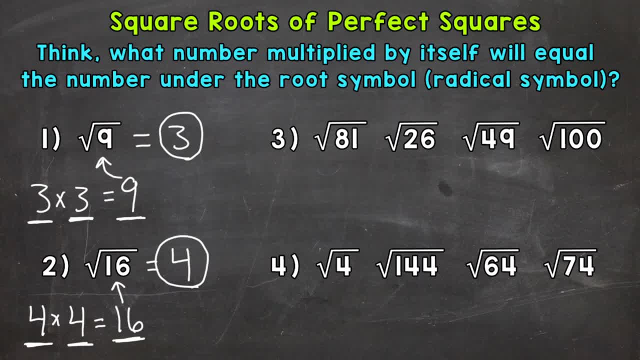 Meaning they have a whole number answer, And 1 will not work out so nicely. Let's solve these and find which ones are the perfect squares and which one is not. So we'll start with number 3.. And first we have the square root of 81.. 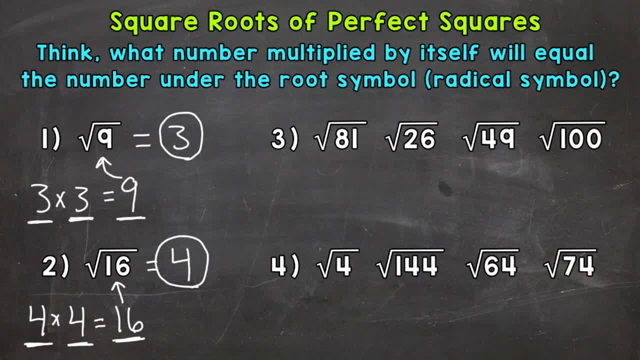 So we need to think any numbers that multiply by themselves to get 81.. Well, 9 times 9.. So 81 is a perfect square. So the square root of 81 equals 9.. So we get a whole number. answer there. 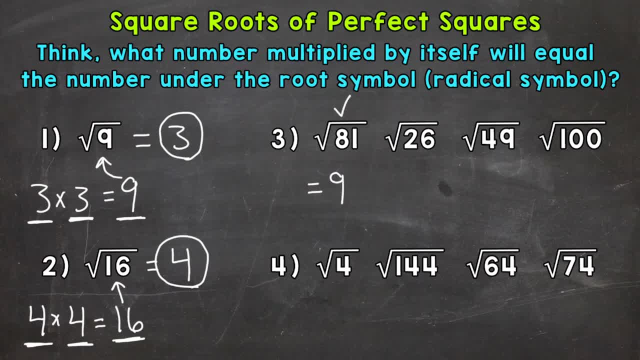 And that is a perfect square, So I will put a check there, Moving on to the square root of 26,. so we need to think any numbers that multiply by itself to equal 26.. Well, we know, 5 times 5 equals 25.. 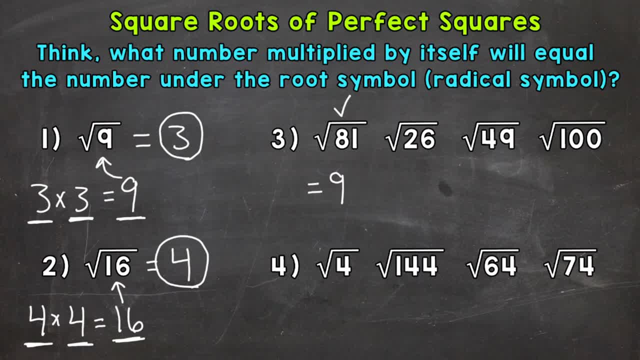 That's close, but not quite. And then 6 times 6 equals 36.. So the square root of 21 equals 9.. This is a perfect square. 26 is going to be somewhere between 5 and 6.. It's not a perfect square and it's not going to give us a whole number answer. 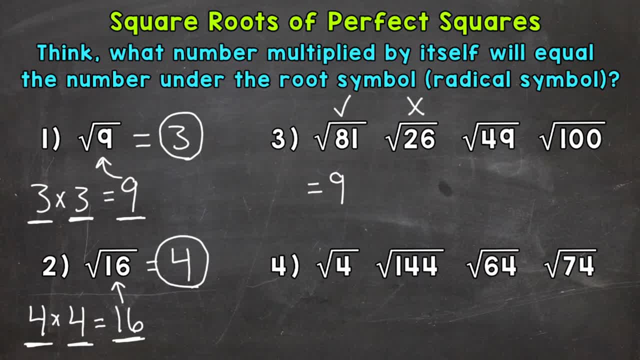 So that's the square root. that is not a perfect square within these four. Let's do the other two, which are perfect squares. So the square root of 49.. 7 times 7 equals 49.. So the square root of 49 equals 7..